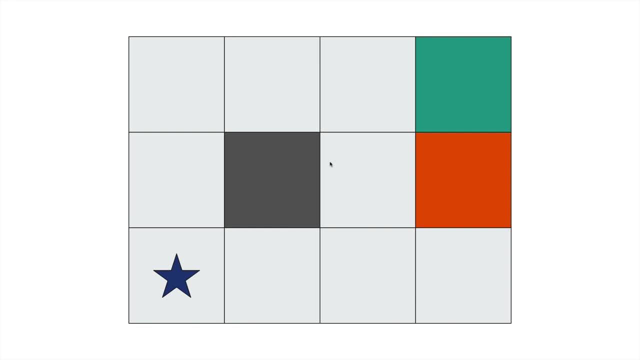 a fire pit that we don't want to fall into. So you know, the goal is we want our robot, which is this little star here. We want a robot to get to the, to find the most efficient path to the green stuff or the green square, the reward, the treasure, And we want to avoid at all costs the fire pit. And one interesting problem here is we're going to make kind of like a real world assumption here is that, in the sense that our motions are 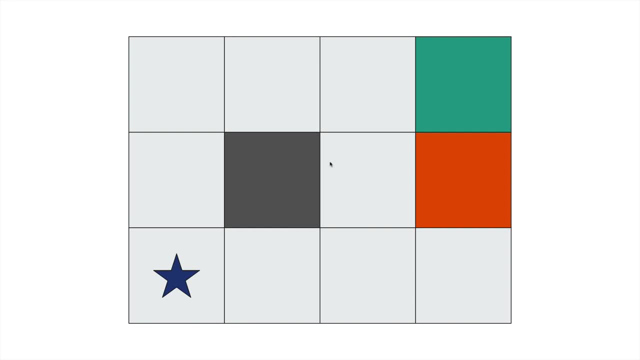 what we call non-deterministic. What that means is if we go to the right, we are not going to go. we might not go to the right, And this, you know, just follow real world assumptions, because if you think of something like robotics, if you try to make your robot move to the left or rotate to the left, it's not going to perfectly rotate 90 degrees to the left. There's going to be some wiggle room here, And so we're kind of also trying to model that in our. we're kind of model that real world, real world assumption into our 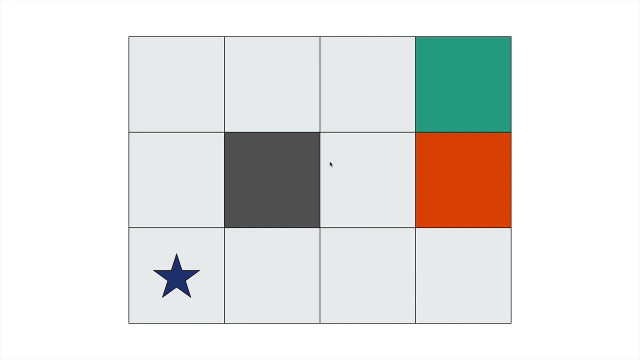 into our reinforcement learning. So when we move, when we say, hey, robot, move to the right, we might not move to the right the entire time, Although there's going to be a very high probability that we do So. maybe, if we say, oh, let's move to the right, maybe there's like a 95 or 90% chance that we do, may take the correct action, But maybe there's a 10% chance that, oh, we like overshoot and actually move to the to, you know, to behind us or down, or you know, there's always that chance. 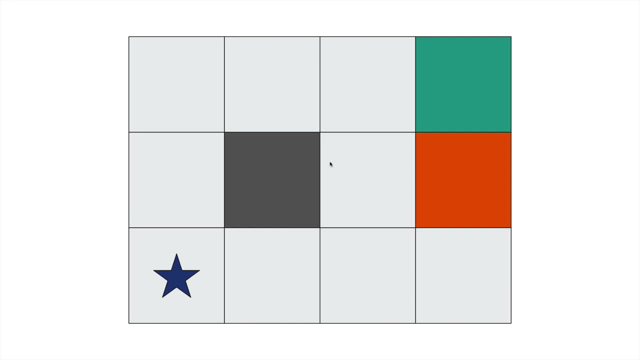 So these motions are non-deterministic, So we don't say move to the right. We don't fully know whether or not it's going to move to the right. We call a non-deterministic, And so the quickest, or objective, is to find the quickest, most efficient path to the goal state. But we don't know what that path really is. And so what we can do is we can try to take moves, And so let me just like try making some moves. So here I'll move to the right, And you know we indeed move to the right. here I'll move to the right. 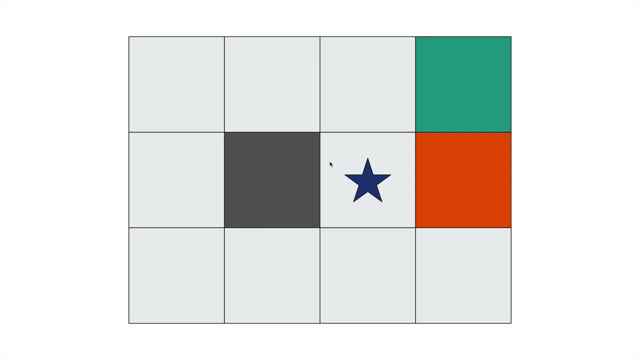 I'll move to the right And then you know, this will work out. And if I keep moving, eventually I'll hit this green state And I'll know that, oh, this is a good reward. I found the treasure, I have a high reward, So this is good. So I've learned that you know, going through this path, this will, this will be good. 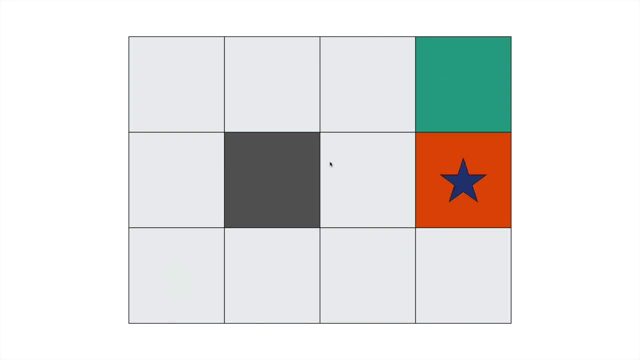 Okay, But now suppose that I, you know, somehow end up in the fire pit. That's not a good reward. And so, as I keep playing over and over again, I'll learn that the green square Is going to be a good reward And the red square is going to be a bad reward. These are things that I might not know at the beginning, But, as I you know, these are what we call end states, which kind of signify the end of the game. 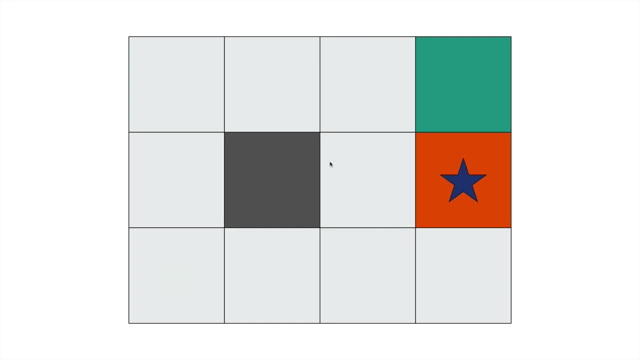 You know, as I keep playing, I'll start to learn where the good rewards are and what paths to take that will get me to these high reward, high reward states. And so here we are back at the beginning, And so we have to kind of formalize this problem a little bit here. 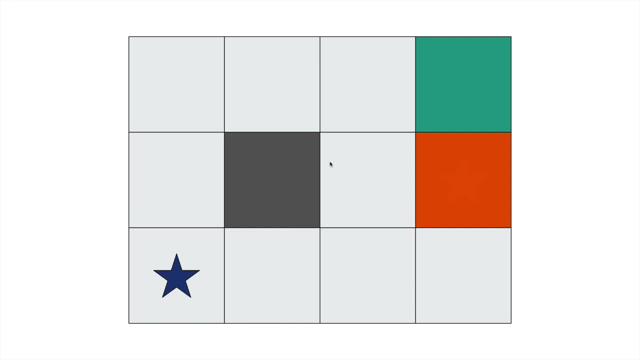 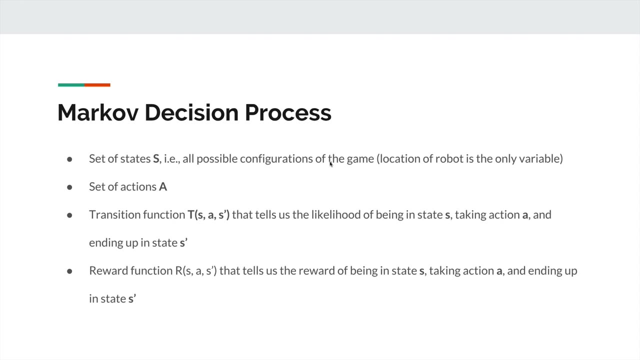 Because if we're going to try to use Algorithms and computer science to kind of solve this, we have to have a bit more of a formal understanding of our problem. And so what we're going to do is this thing called a Markov decision process, And so we're going to discuss these first and value iterations, kind of a way to solve these Markov decision processes, before we get on to, before we get on to Q learning. 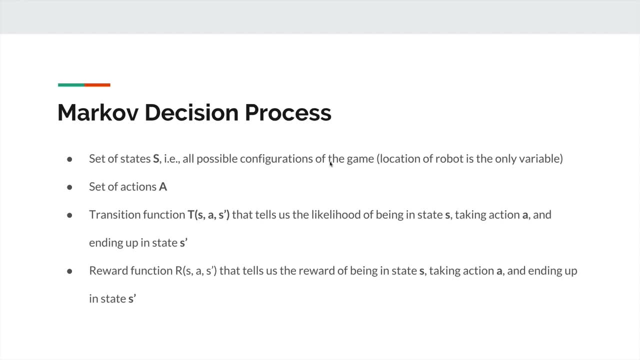 So there are a couple of things that consist of a, of a Markov decision process. So we're going to kind of discuss all of these and then we'll kind of move on to Q learning. This is kind of the formal definition of our, of our problem. 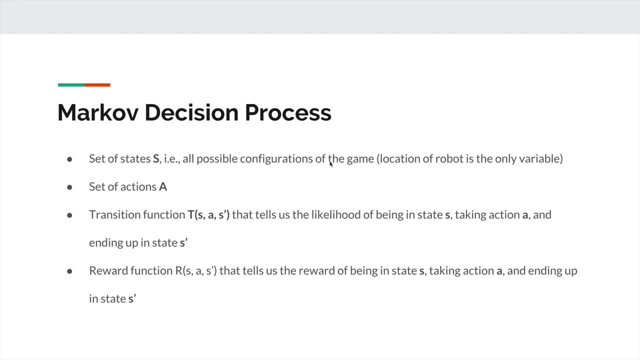 So first thing that we need is a set of states, and a state is just some possible state, represents a configuration of our board, or you know, if we're playing a game of chess, then the state is one possible configuration, And if I move like my, if I move a rook or something, then that just becomes. 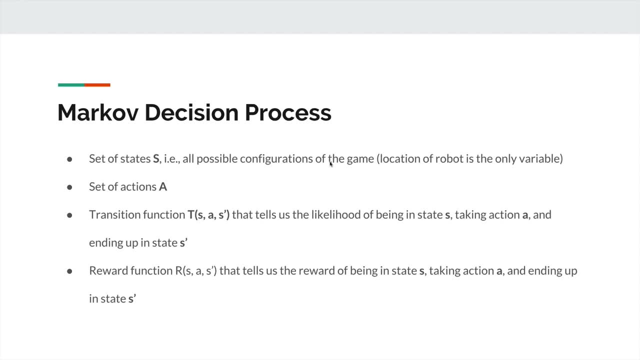 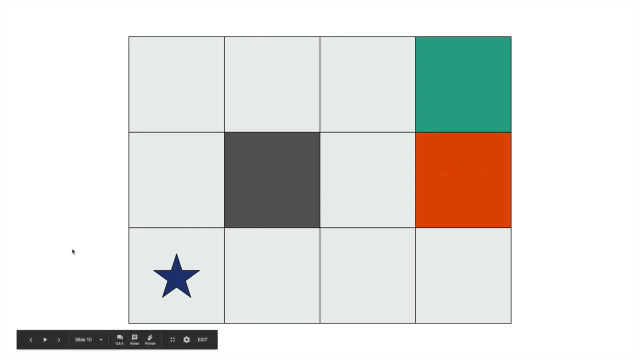 That become a new state. So in the case of our game, the location of the robot is really the only variable. So everything else here is is fixed, except the location of the robot is the only variable. So if I move my robot to the right, that's a new state. 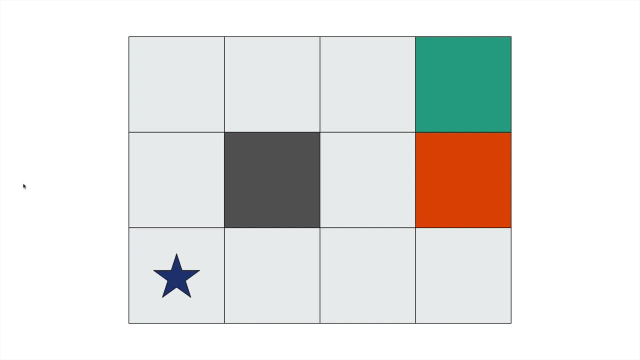 So you can kind of figure out how many possible states there are and just know that in much larger games like chess or something like that, we can have a very, very large number of states. So playing thing, trying to do reinforcement learning with chess, is a bit. 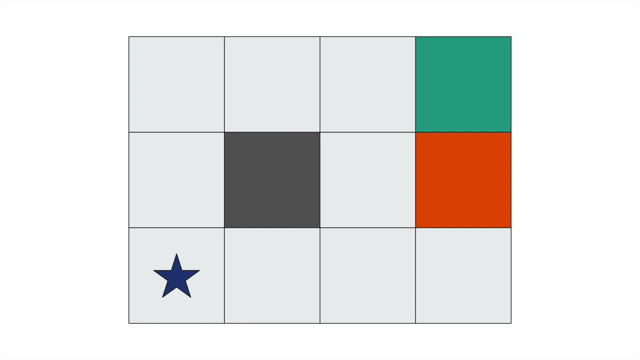 Is it? It's a bit of a challenge and we know there are other ways to, you know, solve this, and then you know that that's. these are just part games. Wait until you get to things like games like Atari games, like you might be familiar with, like missile control or a brick or brick breakout or, you know, Pac-Man or something like that. 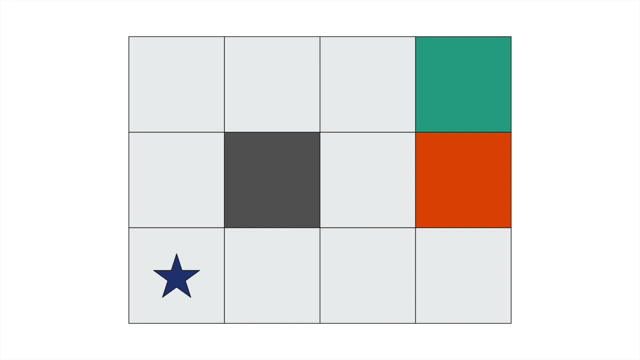 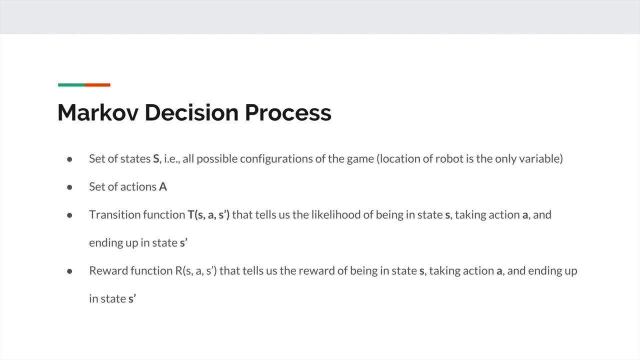 These Atari games they they can have a lot of different states, And so it might not even be tractable to use something like a Markov decision process. but we'll get to that when we get to deep reinforcement learning. But first of all we have to discuss Markov decision processes. 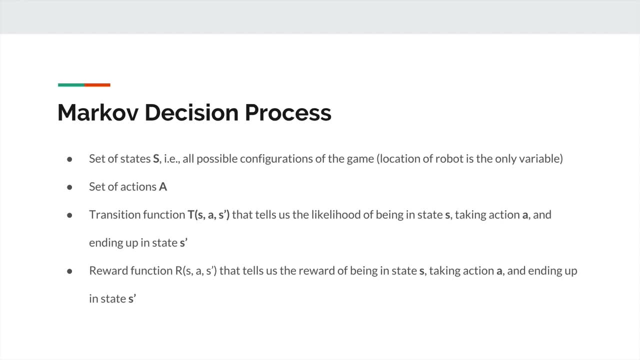 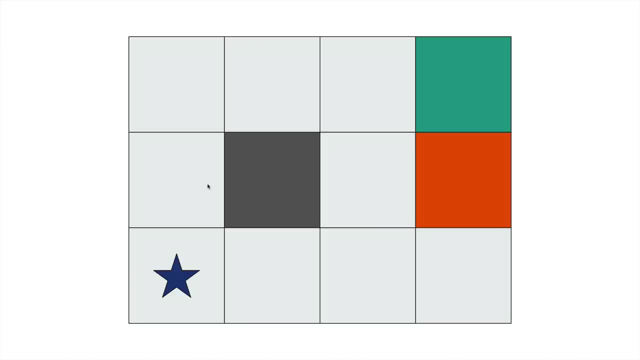 So we have a set of states, And this S? S is all possible configurations of the game. We also have a start state, which is what's the initial configuration here? in this case, for our game, here is the initial configuration. The robot is in the bottom left square. you know, for something like chess we have an initial board configuration. 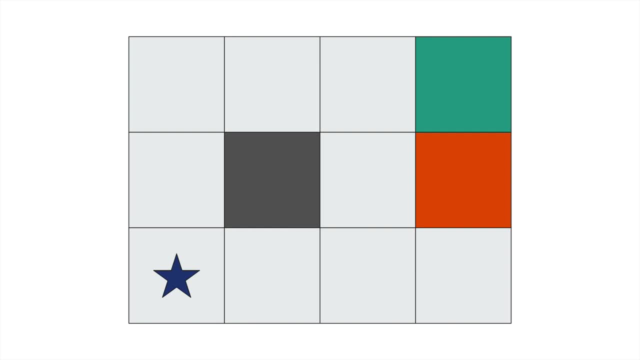 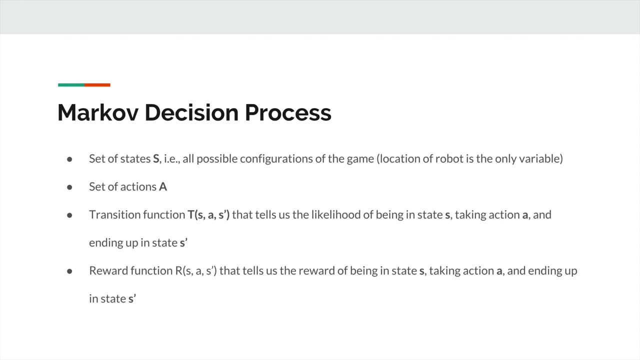 Each piece kind of starts at the beginning. same for Pac-Man. you know, we have all the pellets are there. Pac-Man starts in a fixed spot. each time the ghosts are all in a spot. each time we have some initial state, The next thing we have. 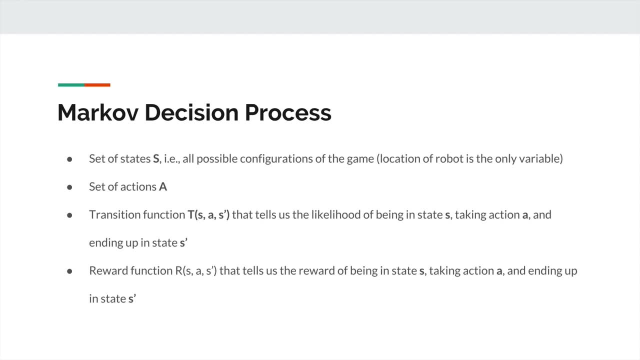 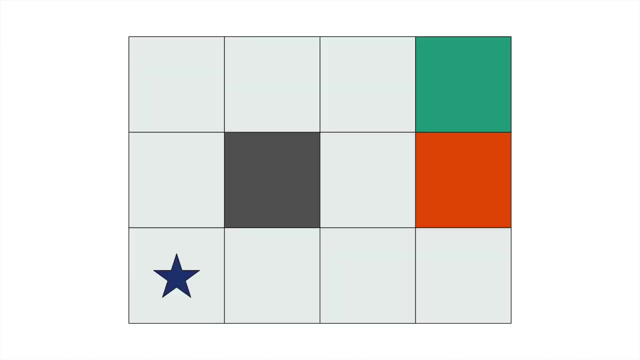 Uh have for um, for a Markov decision process is a set of actions that represents all of the different things that our agent can take And, in fact- and our agent is just something- that our agent is really something that just takes an action in- it's in a particular state and we take an action and then we end up in another state. 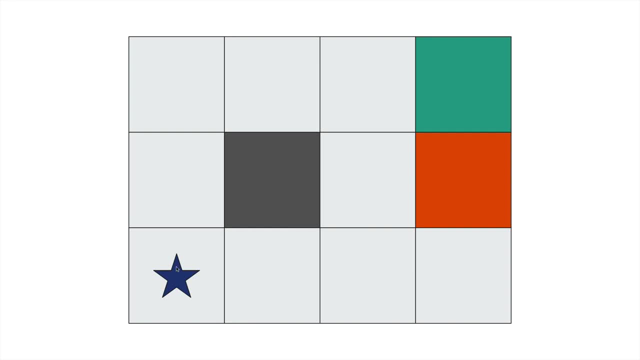 So in this case, our robot is the agent, or whoever's playing the game or a participant of the game. So our robot is um, or what is the agent? And there are a couple of actions that a robot can take. Our robot can go. 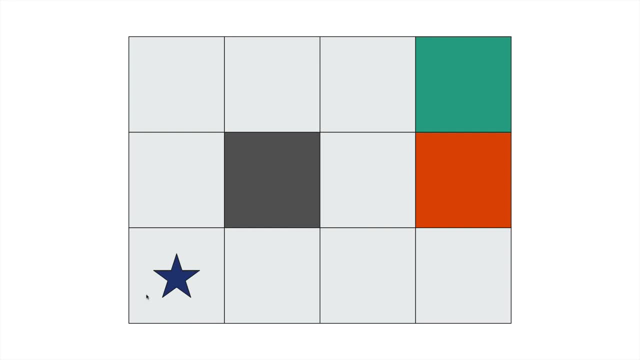 Up. Robot can go to the left, can go to the right and can go down. So those are the possible actions for our robot And maybe we have another action that says, oh well, a robot can just not move Right. 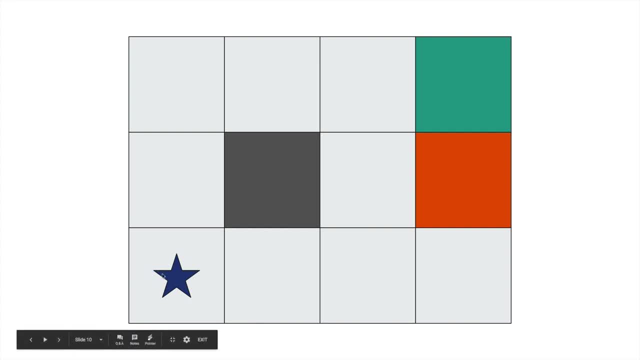 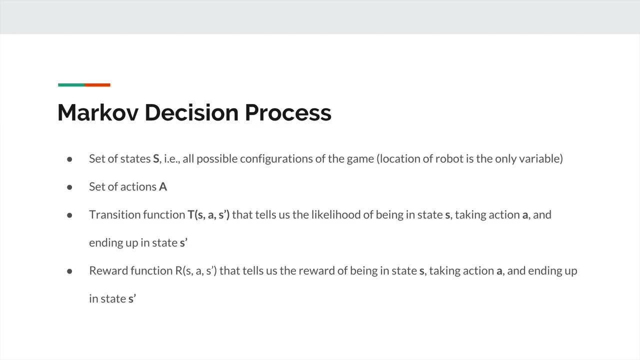 And so we have one, two, three, four, five possible actions here, And you know some games. we might want to make our robot move each time. Our agent movie time, OK, so we've discussed these things and then we have a transition function. 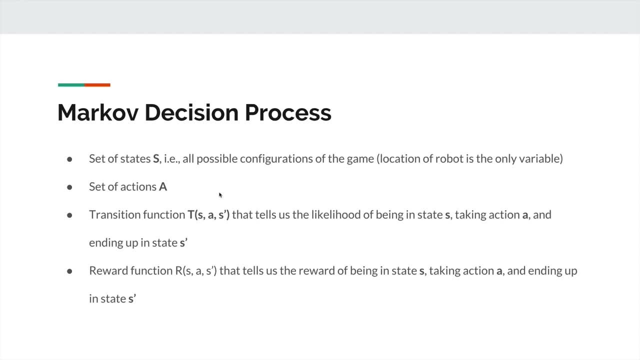 And this transition function tells Us the probability of being in a particular state as taking a particular action, a, and ending up in another state as prime. And the reason that we even have this transition function, remember, is because our environment is non deterministic. 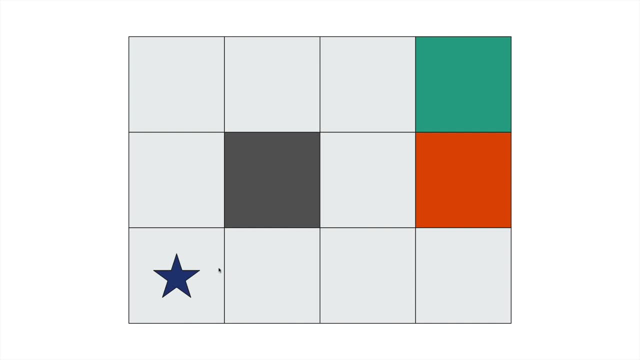 So if I tell my robot, hey, move to the right, there's no one hundred percent guarantee that the robot is going to move to the right. Like I said, it may overshoot or there may be some kind of error, and there's some kind of inherent error in these real world scenarios. 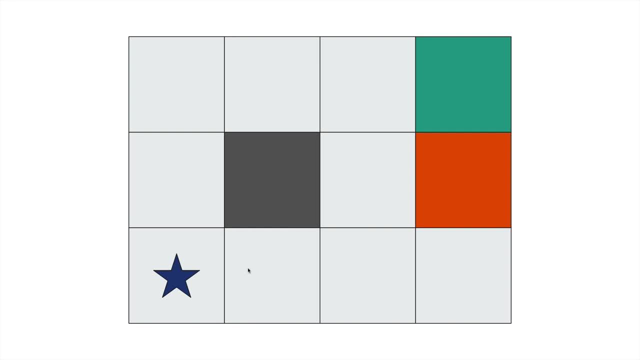 And so it might not always move to the right. So This transition function is trying to encode that. So if I have some state S- here's my state- and my action is moved to the right and I can figure out how many possible ways I can. you know all the possible states that I can end up in. 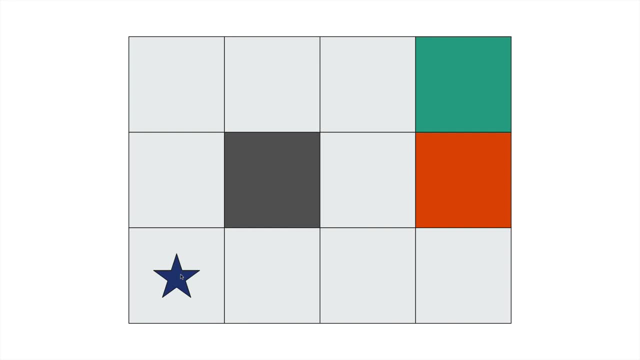 No, there are some other constraints in here, in the sense that a robot can't teleport. We can only move to adjacent states here. So you know, the probability that we're in this state, we move to the right and we end up in the state over here is going to be zero because a robot can't teleport. 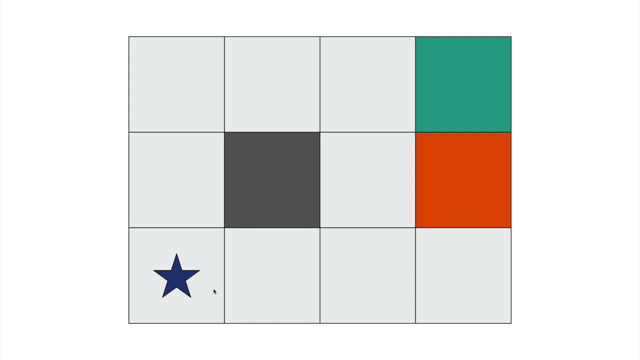 That's another constraint, But you know there are other things that we can do with more realistically. if we had a robot in this scenario and you move to the right, the probability that we actually go right is going to be fairly high, like maybe like 90 percent of the time we actually move to the right. 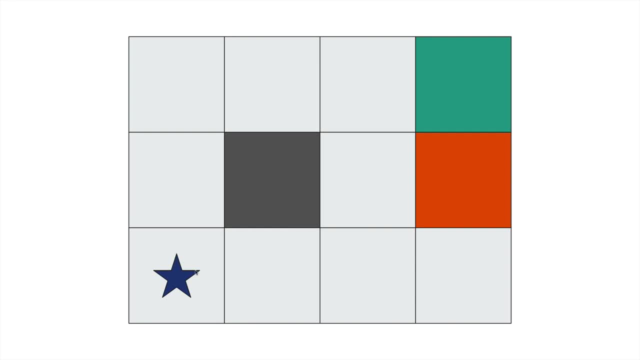 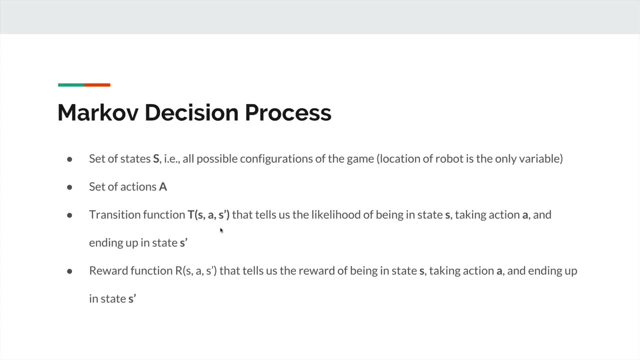 But maybe 5 percent of the time we move up and 5 percent of the time we move down, And so that kind of that transition function kind of encodes that a non determinism in our environment. That's kind of the point of. 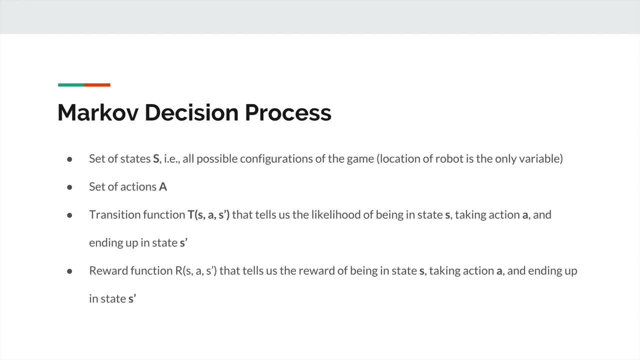 The, the transition function. it's going to become important later on, later on as well, And then, finally, we have this reward function and you see, it's kind of similar to our transition function. So this reward function tells us the reward of being in a particular state, taking an action and ending up in another state. 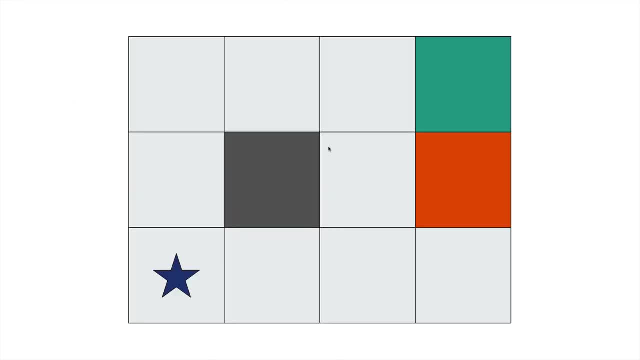 And this is a reward and kind of the whole goal is to maximize our reward. And so if I were, instead, if my robot were in, let's go back here. All right, My robot were in this state, Here's my state s, and I go to take to the right and I end up in this green square. 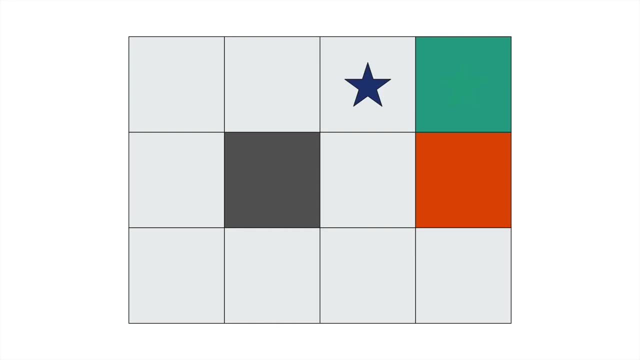 Then I'm going to have a high reward, And that's exactly what I want. That's what my reward function is going to tell me. But instead, if I end up in this state here, I'm going to have, like, maybe, a negative reward. 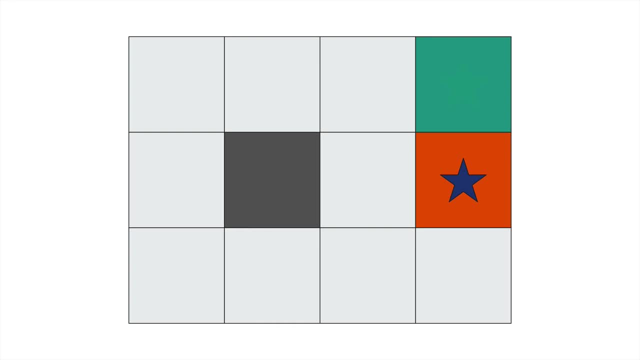 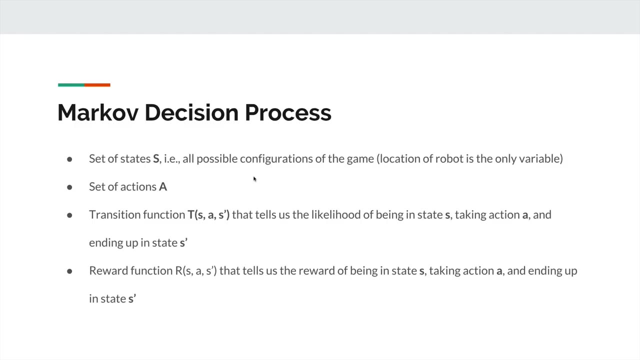 And that's going to be very bad. And so the reward function is what we're going to use to kind of figure out what states are good and what states are bad. And so we know all of this information- Actually we know all of. 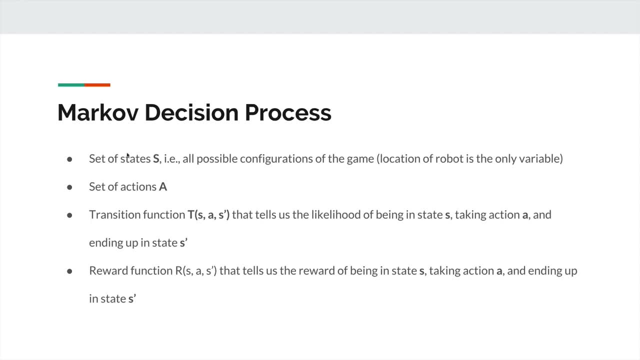 This information, we know all the possible states, we know the initial state, we know all the actions we can take, We know these probabilities and we know the rewards, And so we have all of this information at our disposal, And so now we can start building algorithms around this that you know, that can help solve our problem. 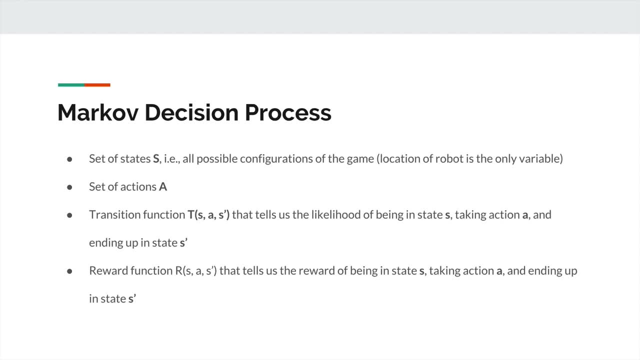 We want to get. we want to figure out where the high reward states are and find the most efficient path to them. So another kind of key word I want to explain before we wrap up Is: the goal is to find what's called an optimal policy. 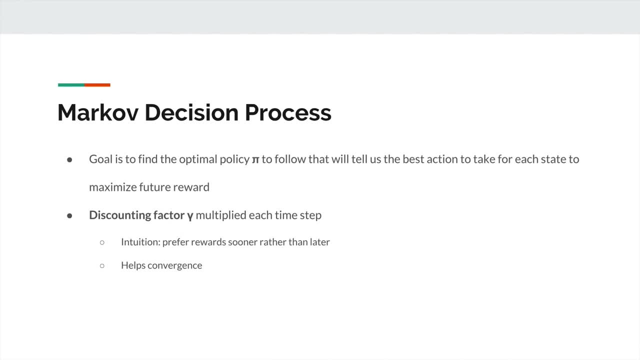 And the policy essentially just tells us which action to take in a particular state that will lead us to the maximum reward in the future. So what? the policy is just a function of the state that we're in. So let me give you- let's go back here to do another example- 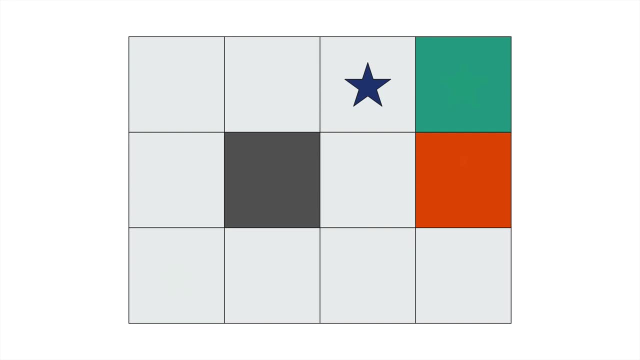 So if we're in this state, the policy, if we, after we've trained a reinforcement learning agent, the policy will say, hey, go to the right, And that will give us the maximum reward, You know. and the policy, if we were in this state, the policy would say, hey, don't go up, or go up and don't go to the right. 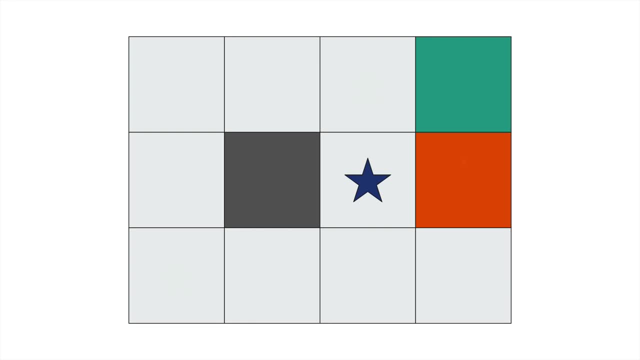 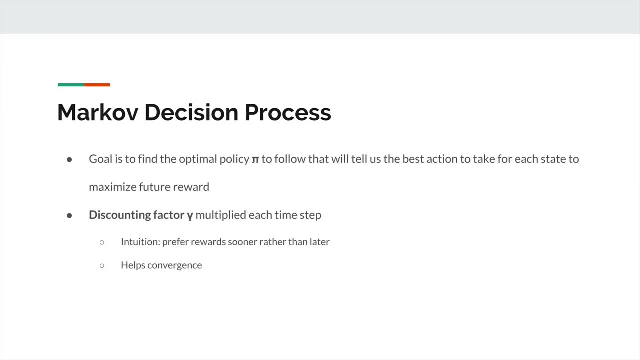 And that will give us that will end up with the maximum future reward. And so you know that's what the policy and the whole goal of reinforcement learning is. to figure out this policy, We kind of go over here. So the goal is to find that optimal policy that will tell us take the best action to take. 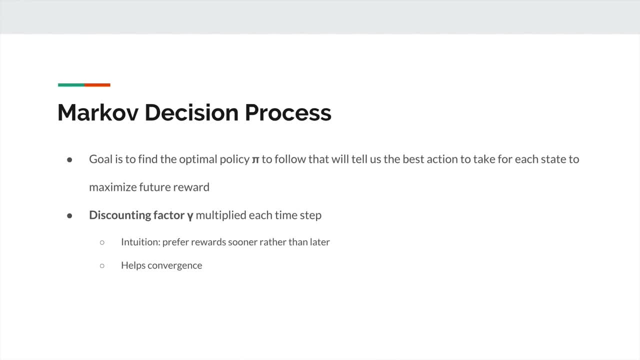 And one other thing That I want to discuss real quickly is this thing called discounting, and that's denoted by the sex of the Greek symbol, gamma, And at each time step we have this notion of discounting and kind of the intuition behind this is that we prefer to have rewards sooner rather than later. 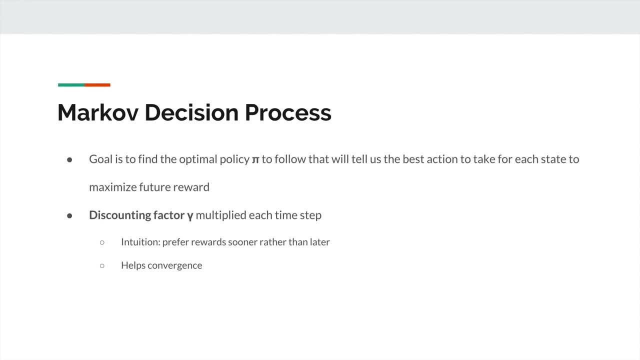 And you'll see that when we get into the actual value iteration algorithm, this discounting factor is actually kind of crucial, because it helps our values, our expected rewards, converge, And so we know which is the best path to take, And so we have this kind of notion of